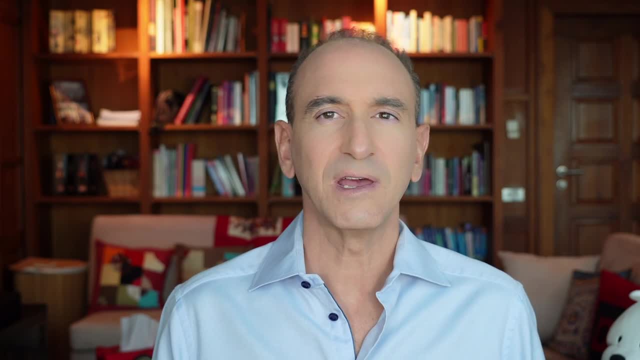 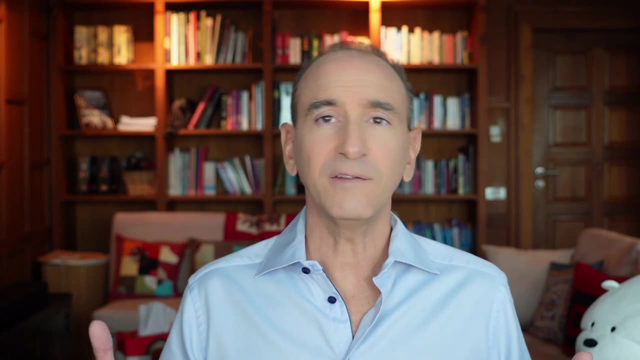 known for its strengths and that has gone hand in hand with the economic development of Singapore. But how about the Singaporean dollar, if you would take an investor perspective? So I did the research and the math and, looking back at January 1st 2000 as a starting date up until 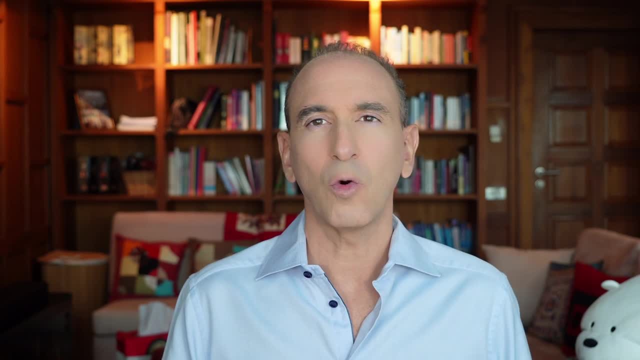 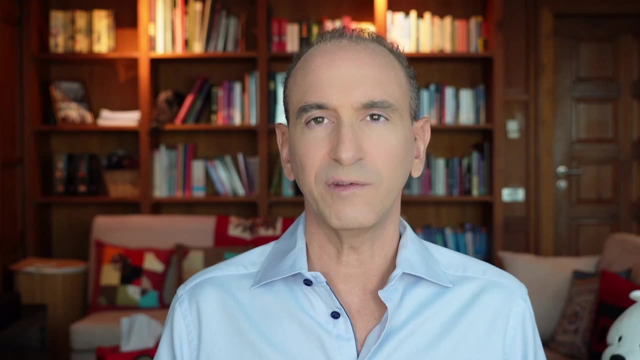 31st of December 2021, to look at what is the best currency And, as before, I'm doing a comparison with the US dollar, because it's a very strong currency and it's also the reserve currency in the world: US dollar or Singapore dollar? Who is the winner of the boxing match? Let's find out. 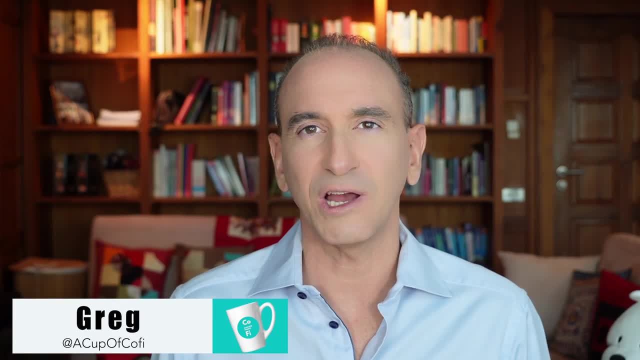 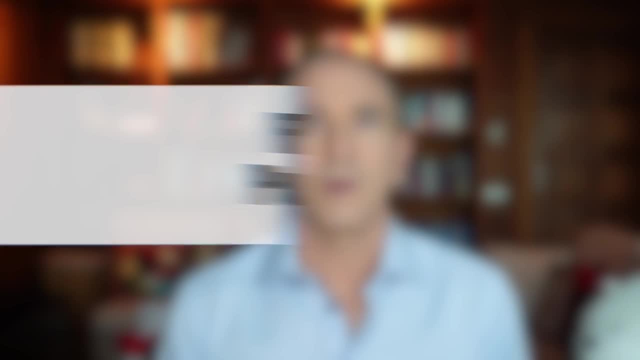 My name is Greg Angelbert. I'm a life and personal finance coach. I share what I know about coaching and personal finance on a cup of coffee. In this video, I'm going to talk about what is the best currency to help you live a life of. 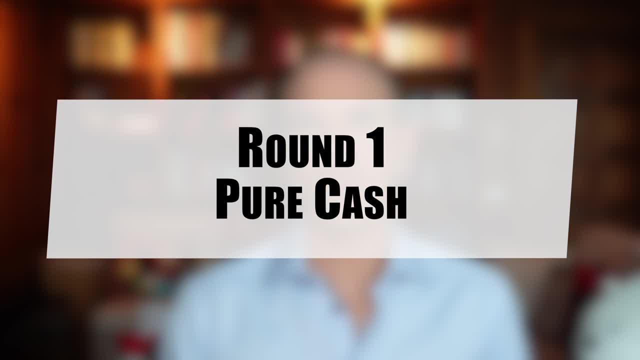 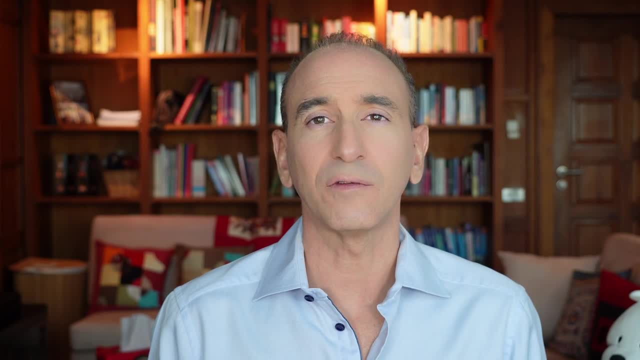 purpose and build up your wealth Round one: pure cash. With the current level of inflation, keeping cash in the bank might seem to be a way of losing your purchasing power pretty much every day. Having said that, if you look at the returns of the stock market since the beginning of 2022,. 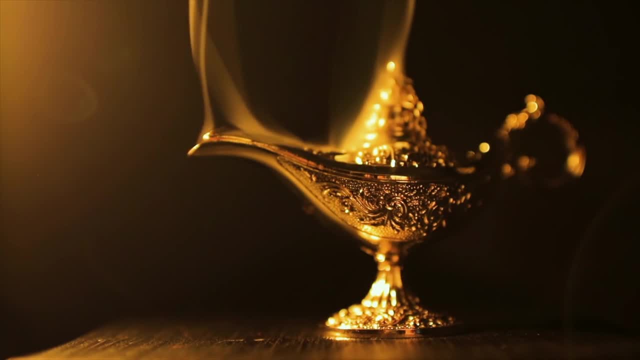 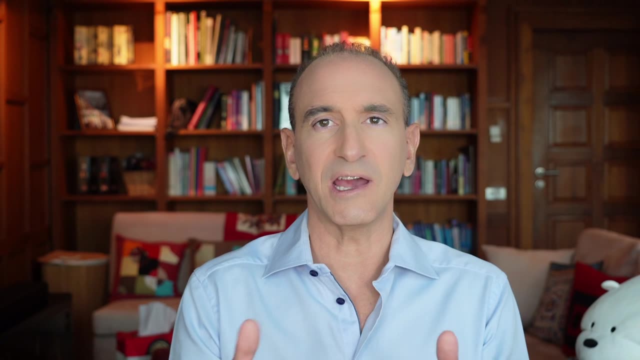 then you might get a very different picture. Let's imagine that on the 1st of January 2000,, a genie just appeared in front of us and gave us 10 000 US dollars, But the trick was that we had to put it uniquely in cash, which is a good thing. So let's get started. 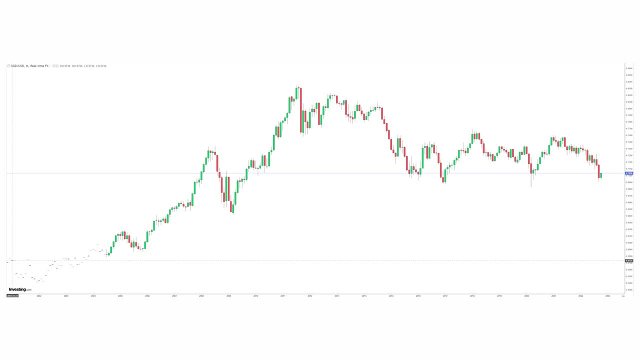 We have to keep it in cash And we have to keep it, whether in US dollar or Singapore dollar, for 22 years. Considering that you can see the evolution of the Singapore dollar versus US dollar from 1st of January 2000 to 31st of December 2021. That is not a pretty picture. for US dollar. If you would look at it for 2022, it looks a bit better for the US dollar. 10 000 US dollar on the 1st of January 2000 was converted to 16 565 Singapore dollars. 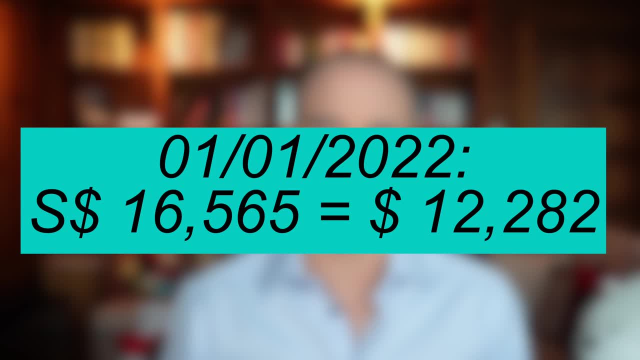 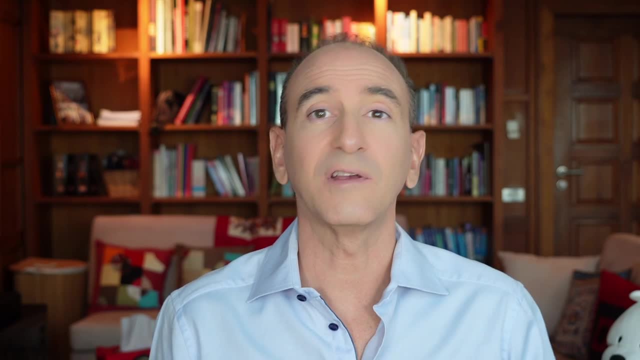 On January 1st 2022,. we converted it back into US dollar to compare with the original investment of 10 000 US dollar And we get 12 282 US dollar. Clear here: the Singapore dollar most definitely win Additionally over this period. the consumer price index, the CPI, a measure of inflation, rose by 42.1% in Singapore. In the US, the CPI rose by 62.7%. Considering that the US and Singapore are two rich countries, we can roughly estimate that they would have the same basket of consumption for citizens. 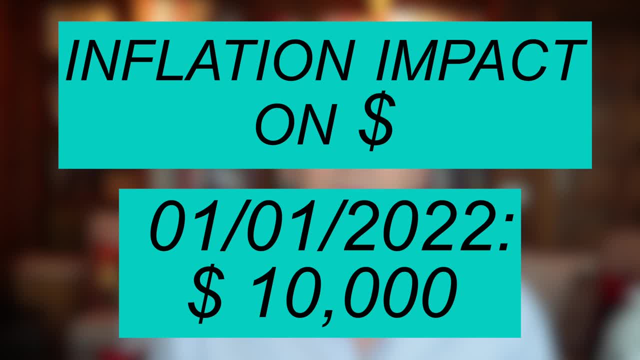 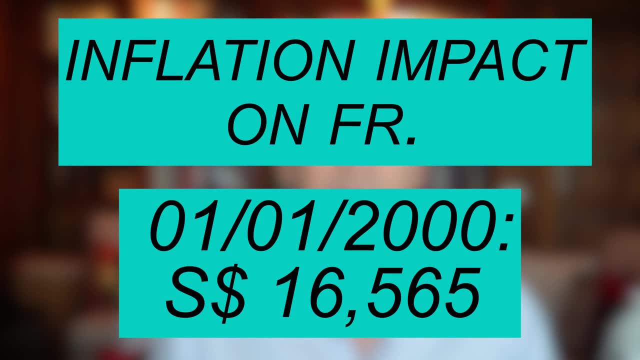 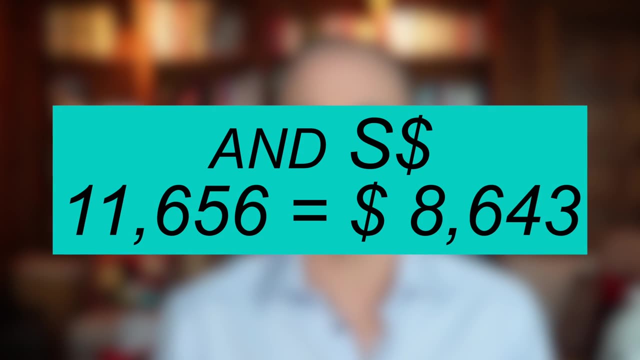 of each country. So the 10 000 US dollar have devalued to purchasing power of 6146 US dollar today, compared to 2000.. The 16 565 Singapore dollar have devalued to 11 656, which translate into 8 643 dollars, 8 600 versus 6 100. the Singapore dollar still wins. 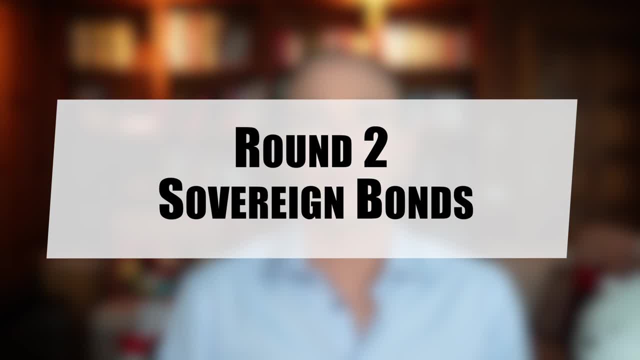 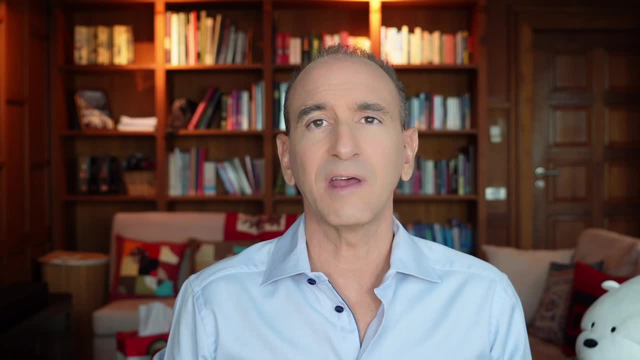 Overall. round one goes to Singapore. dollar Round two sovereign bonds. Now the genie changes his mind and tell us that we need to take those 10 000 US dollar and invest them in 10-year sovereign bonds, whether from Singapore or from the US. He's. 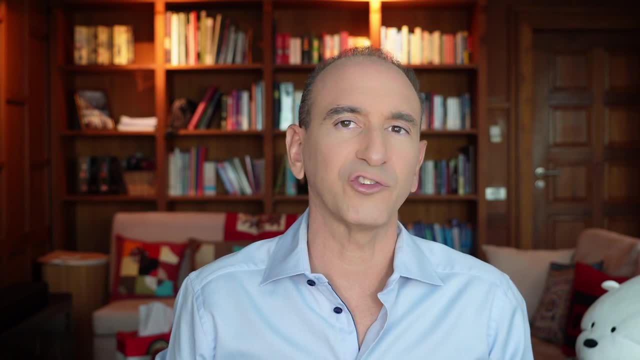 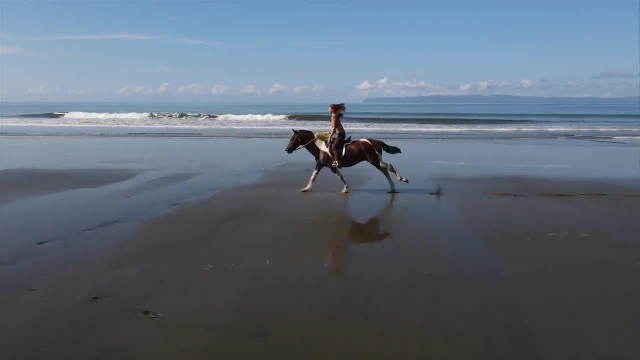 being nice with us and believes that it's going to be a better return than pure cash. We assume here buying and selling the bonds beginning and end of the year so we can ride the evolution of the 10-year bond year by year. The bonds are the federal reserve bond in the US. 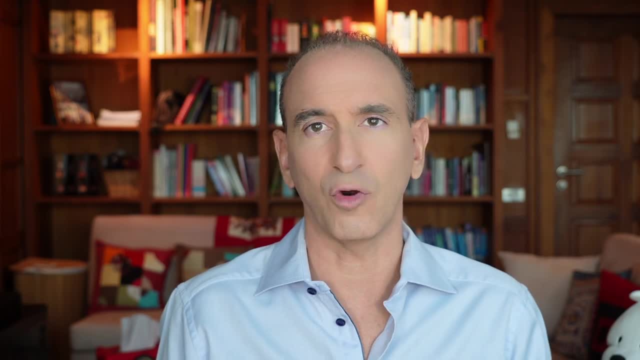 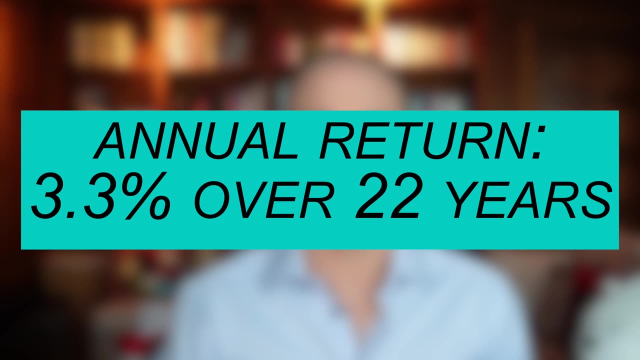 and they are the bonds from the monetary authority of Singapore. Our 10 000 US dollar would become 19 908 US dollar by January 1st 2022, which is almost doubling our investment amount And, as you can see, the 10 000 US dollar is a 3.3% yearly increase over the period. 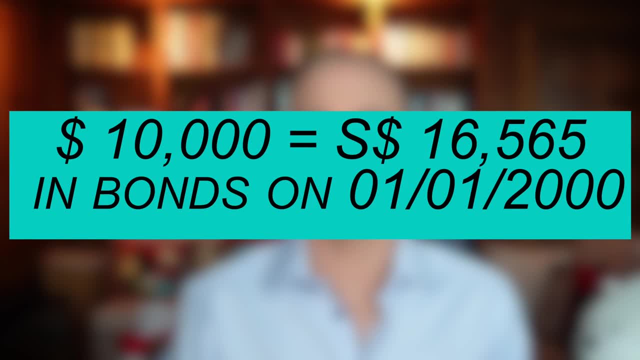 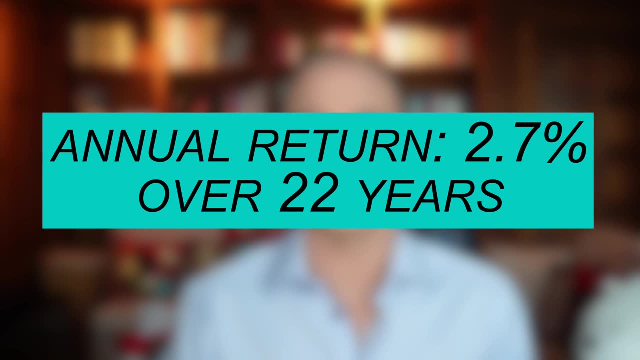 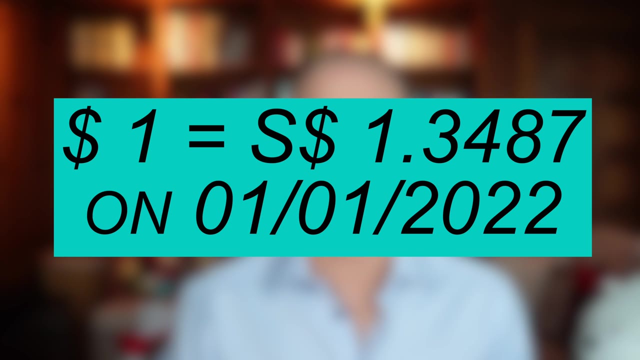 If we look at our 16 565 Singapore dollars, they would have become 28 786 dollars, which is a 74% increase, or 2.7% nominal return per year, Though we need to compare it to its dollar equivalent. so we use the exchange rate of January 1st 2022, which is 1.3487 Singapore dollar to the US dollar. 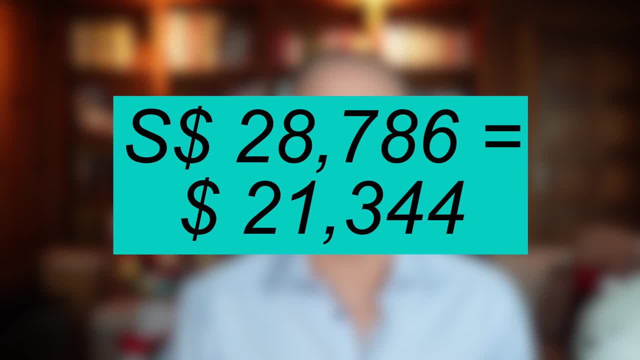 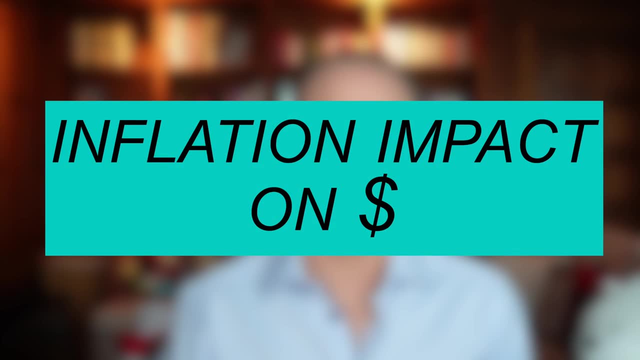 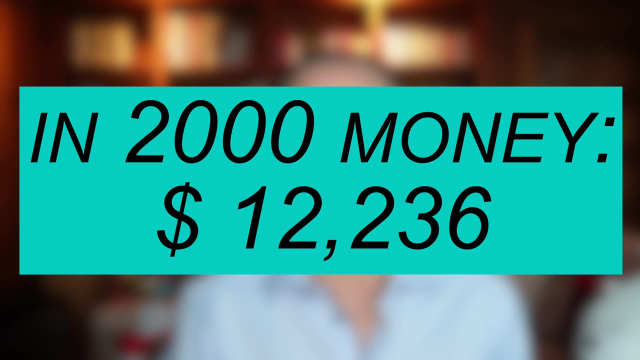 We then get 21 344 US dollar which, compared to the 10 000 invested originally, gives us a 3.7% annual return over the period. Taking inflation into account, as per the cash calculation, the 19 908 US dollar are effectively devalued to 12 236 US dollar. if you had stayed with your money. 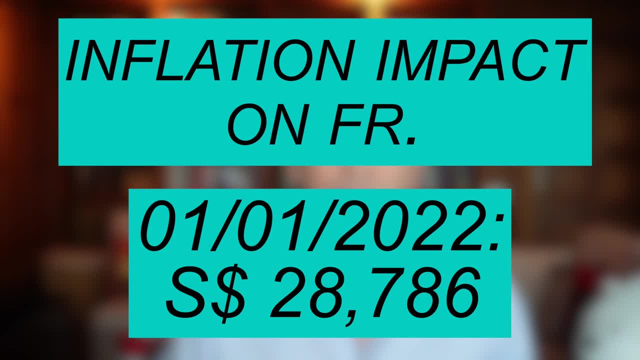 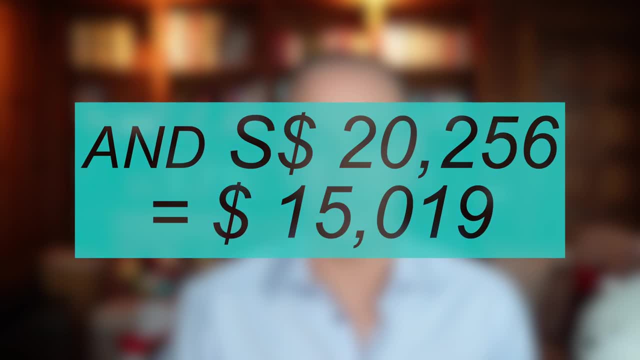 in the US, The 28 786 Singapore dollar would have devalued to 20 256 dollar, which is the equivalent of 15 019 US dollar. 15 000 US dollar versus 12 200 US dollar. the edge is for the Singapore dollar. 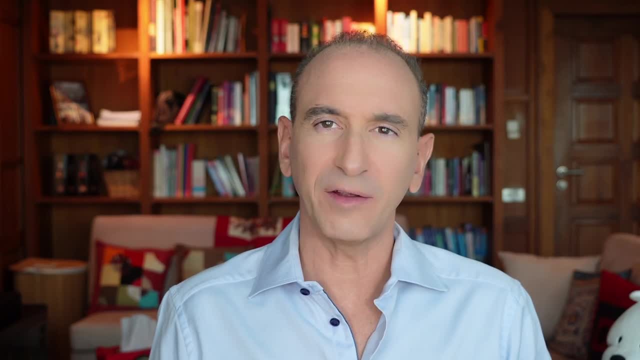 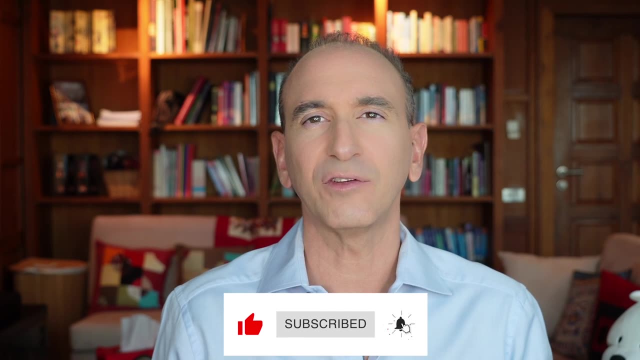 The winner of this round is clearly the Singapore dollar. Do you like this comparison video between the US dollar and Singapore dollar? Though you know what to do and also subscribe to the channel and put the notifications on if you want to receive content like this every week. Also check out other videos from youtubers. 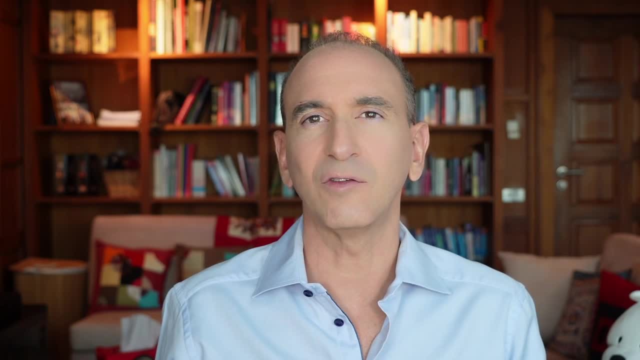 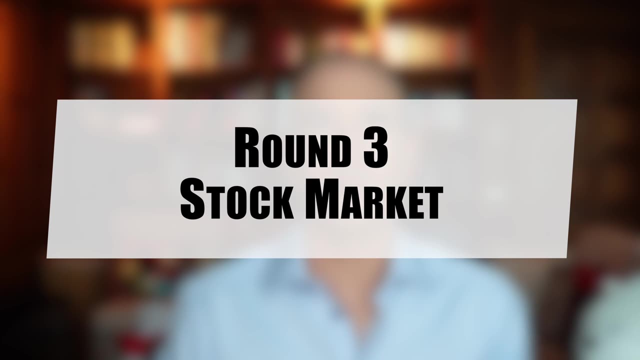 which you can find in the description. it's interesting and important that you look at different point of view about this topic. Round 3, stock market. The genie is now going full tilt and tell us that we need to invest our 10 000 US dollar. 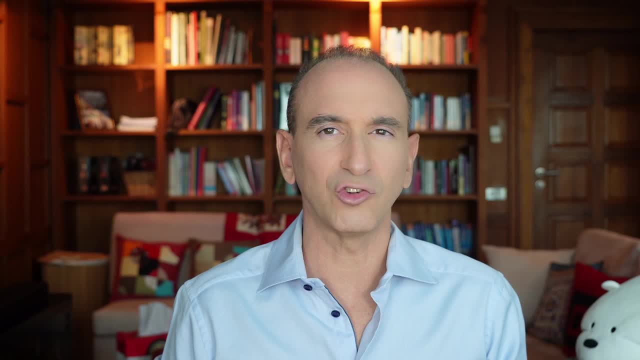 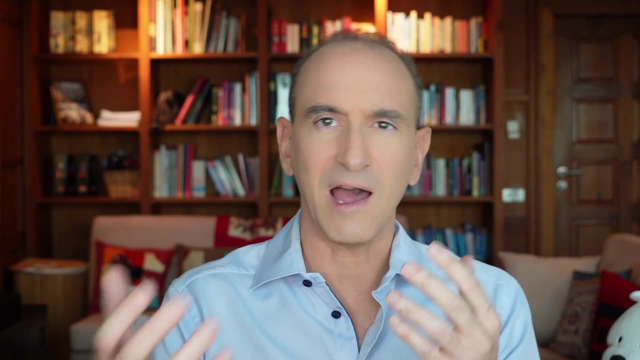 in the stock market, And to do that we do not have to take a lot of risk. we can just invest in the top companies in the New York stock exchange and also in the Singapore exchange. The two indexes that we can have from both countries are: first, the Dow Jones industrial. 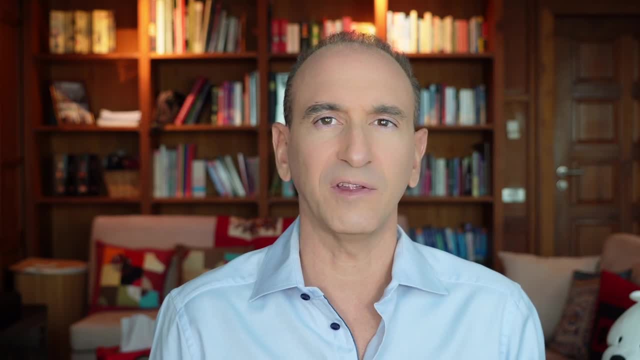 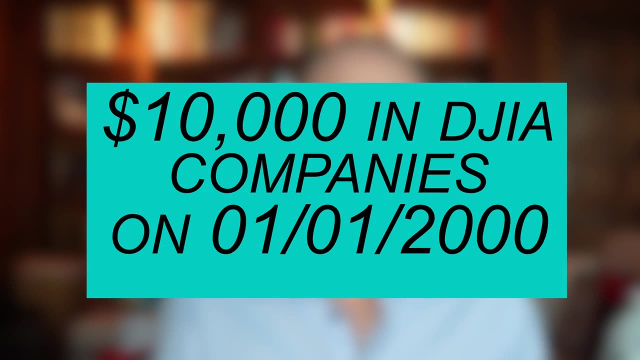 index in the US for the top 30 companies for market capitalization And for Singapore we can take the Straits Times index which also represents the top 30 companies by market capitalization: 10 000 US dollar investing on January 1st 2000 in the Dow Jones industrial index and rebalance. 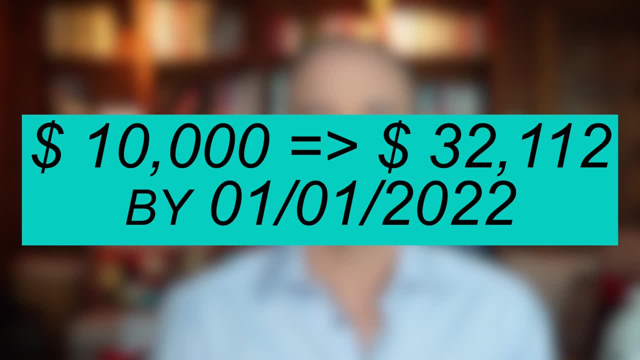 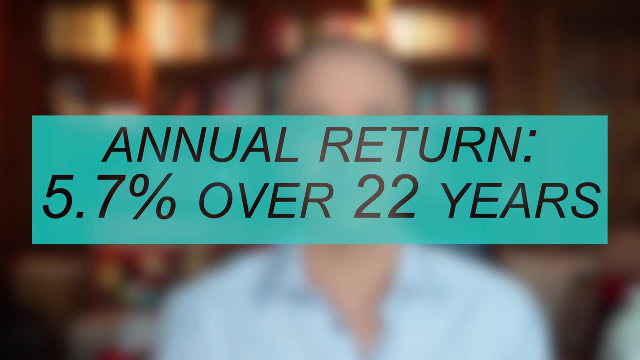 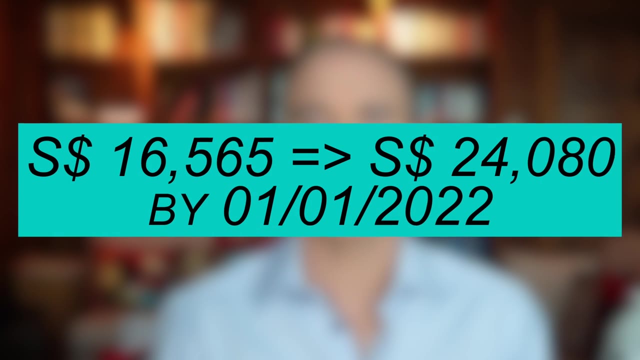 continuously to follow it until January 1st 2022 would have increased to 32 000 US dollar, Which is more than tripling and an annual return of 5.7%. That's okay. Our 16 565 Singapore dollar invested over the same period in the STI in Singapore and rebalanced continuously, would 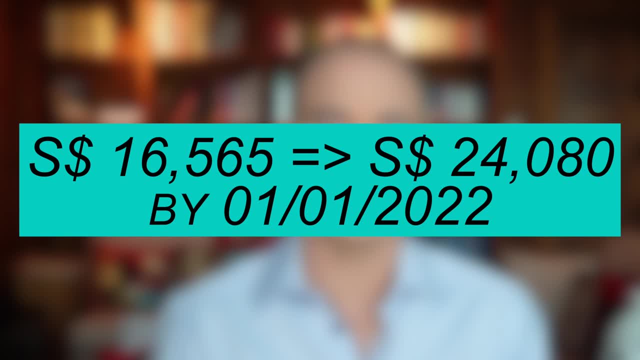 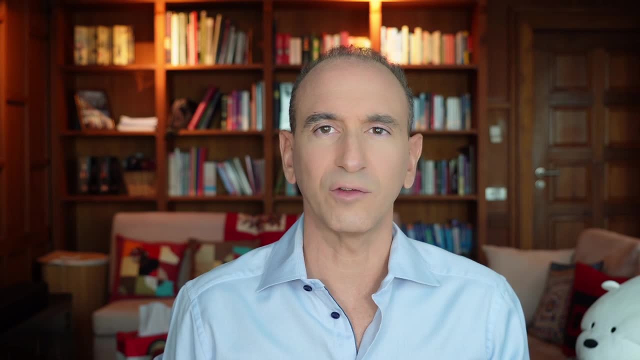 have increased to 24 080 Singapore dollar, which is a 45% increase or 1.8% annual return. Not good. Let's see how it compares when we translate that to US dollar. We get 17 855 US dollar for 24 080. 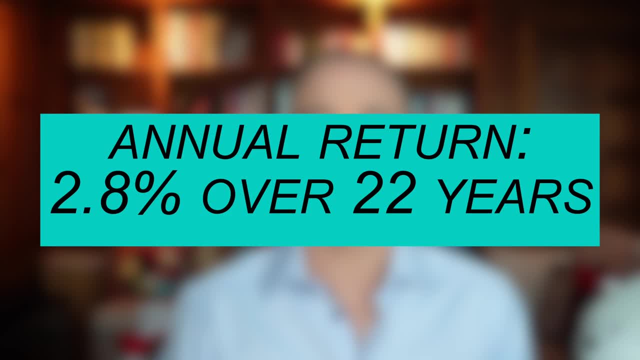 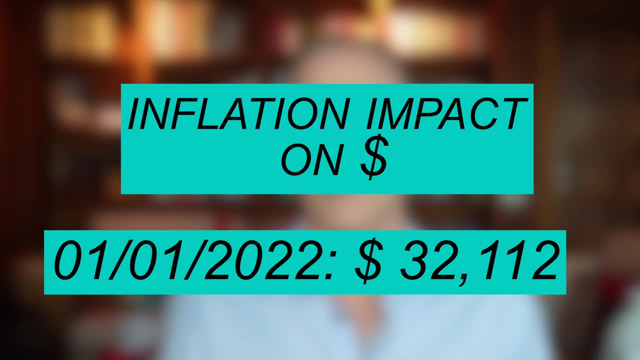 Singapore dollar, which gives us a net annual return of 2.8%, based on 10 000 US dollar invested. That's better, but that's still not good. Taking inflation into account, the 32 112 US dollar invested in the US are effectively. 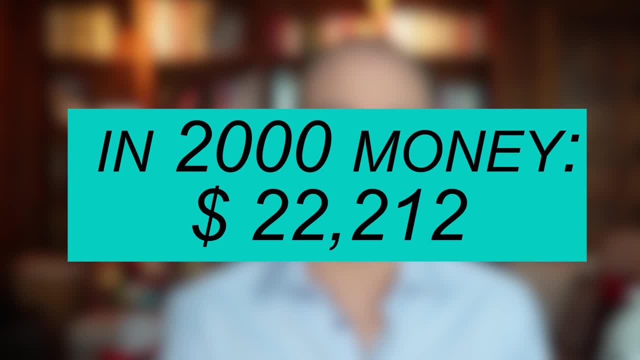 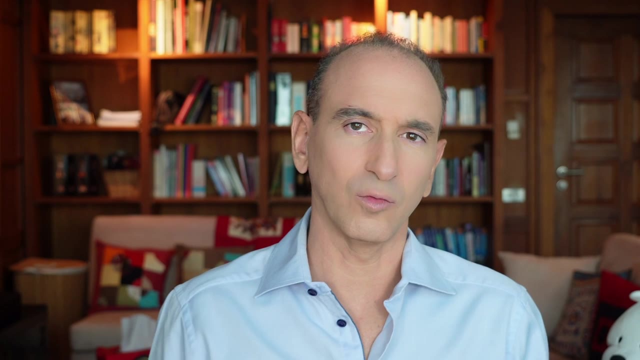 devalued to 22 212 US dollar. if you had stayed with your money there, The 24 080 Singapore dollar would have devalued to 16 945 Singapore dollar, which is the equivalent of 12 564 US dollar: 12 500 versus 22 100. 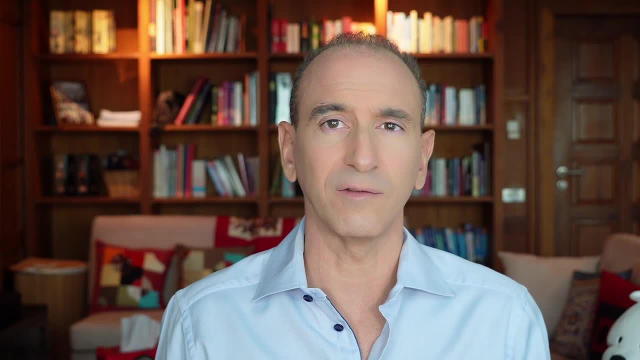 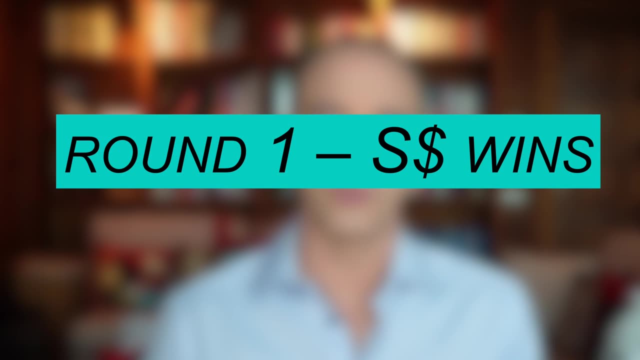 US dollar is a massive gap, which is to the benefits of the US dollar investing in US stocks. The USD is a clear winner of this round And the winner is- Let's look at the summary here. Round 1: staying in cash goes to the Singapore dollar. Round 2: investment with sovereign bonds. of the respective countries goes to the Singapore dollar. Round 3. investment in core companies of the US or Singapore goes clearly to investment in the US. If you had planned to have some of your money invested in sovereign bonds, then you should definitely have gone for the Singapore dollar of the past 22 years. 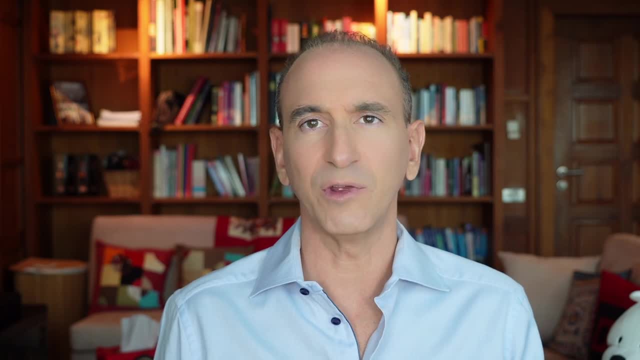 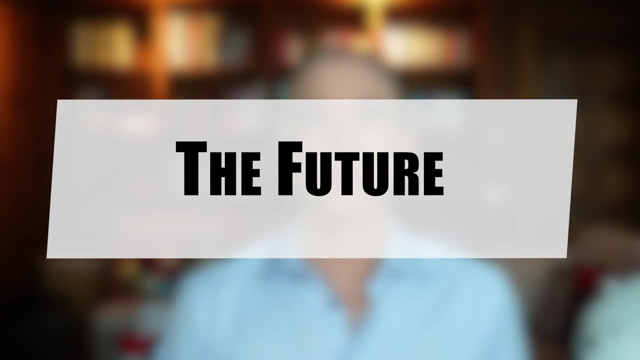 But if you wanted to take more risk and actually have a better return on investment, it's quite clear that the US dollar with US stocks, would have much better performed. The future: We're moving on from our genie now to a divining spirit. The future depends on two main things. On one side, it is a 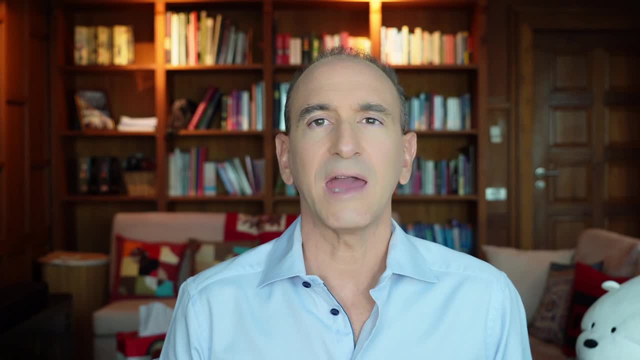 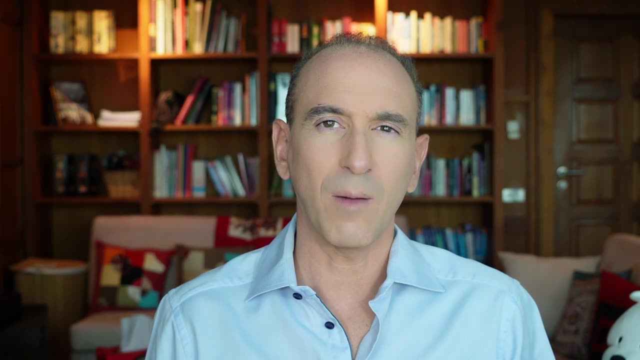 return of cash stock bonds and on the other side, it is the evolution- the future evolution, of the exchange rate between the Singapore dollar and the US dollar. The bonds for the US and Singapore are a trend over the next 10 years to be at the same level because they have actually converged over. the past 10 years. Regarding stocks, the US stock market is much more vibrant, alive, than the Singapore stock market, simply because there are a lot of companies coming in and out. There's a lot more companies in the US than there are in Singapore: 50% of the straight times index. 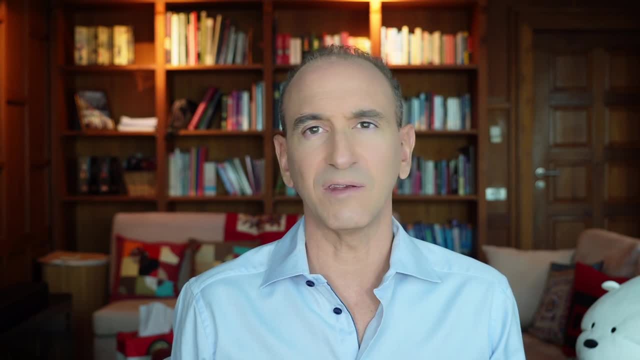 in Singapore is dependent upon household names which have been there for quite a while and which are quite stable, like DBS, UOB, OCBC, Singtel and Charlene Matheson. All of those stocks are in banking or the mature industries which are not growing very fast. The other factor to take into account is the exchange rate, and that very much depends on the policies of the Fed in the US and the Singapore Monetary Authority. The Monetary Authority of Singapore has a primary mandate of trying to keep the exchange rate not moving too much. 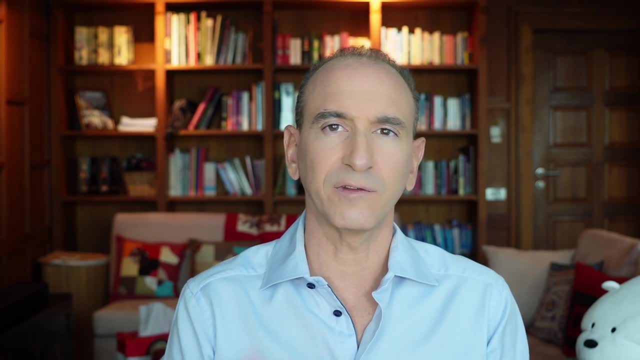 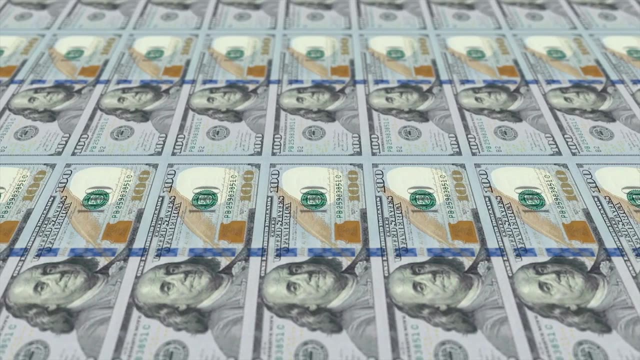 particularly with regards to the position of exports and imports in the country, because Singapore is an export economy. For that it's using its close to 300 billion US dollars of reserve currencies to be able to intervene in the market in case they want to see the Singapore. 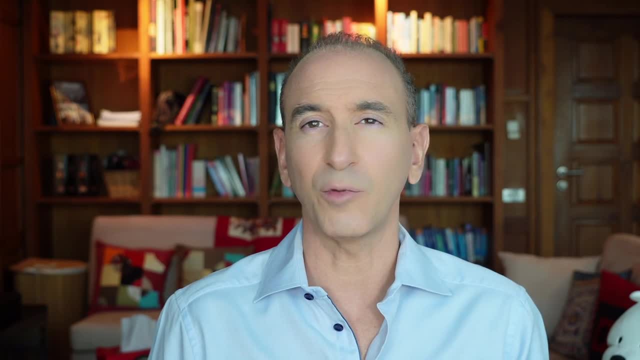 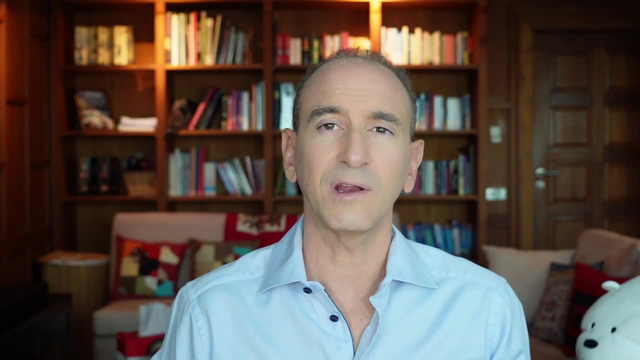 dollar going up or down. They also rely on the strength of the economy and the perception of that strength from international investors. And the value of the Singapore dollar also depends, on one side, on the economy, as we said, and on the other side about the size of the assets that 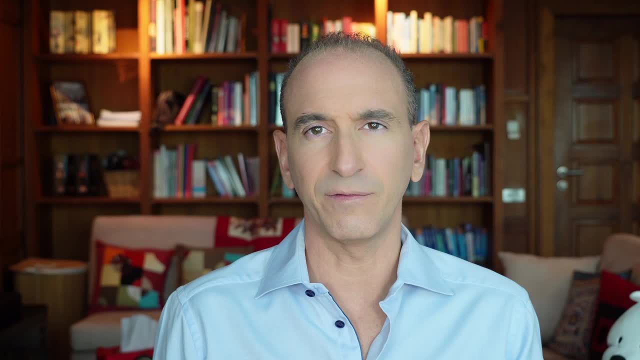 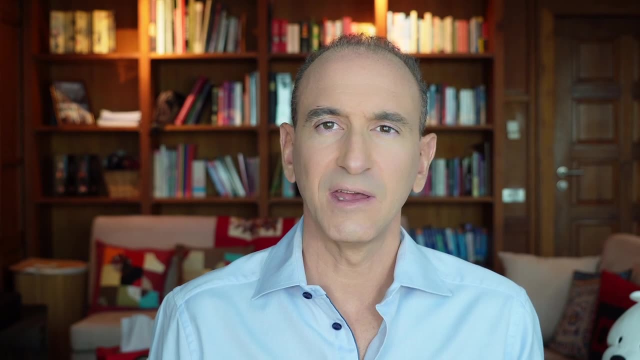 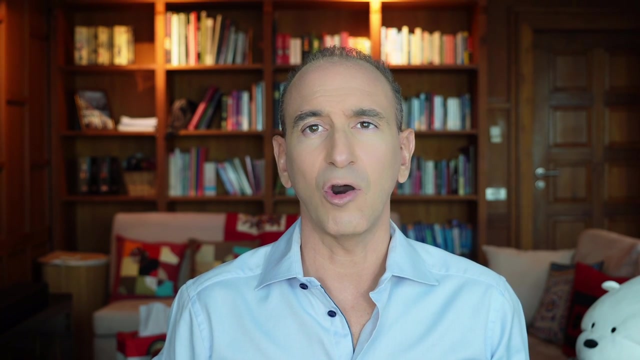 Singapore has With two very large sovereign investment funds, GIC and Temasek, which represent Singapore has a very strong financial position in terms of assets that it's managing and owning. For the US, the Fed has a mandate of making sure that inflation stays about 2% per year. 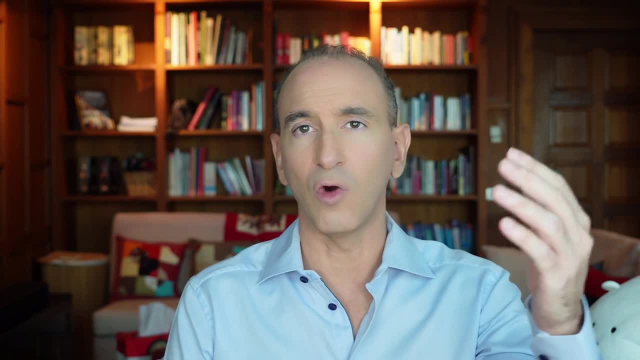 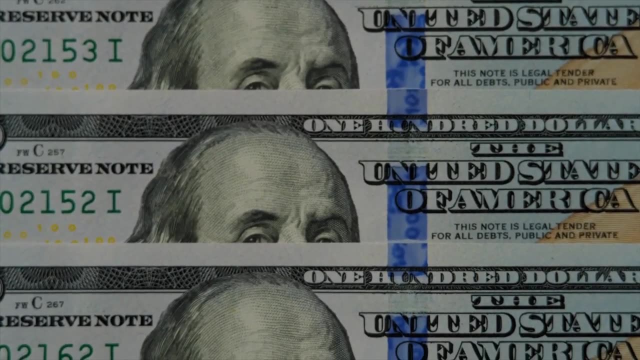 and also that the Fed will support economic activity not too high and not too low. The US has the enormous advantage of having the world reserve currency with the US dollar. that allows them to basically support economic growth with printing more money. But the party must end.